minus b. So this is true. This is eternal. Now you should be able to calculate, In addition to which we can substitute the home away from apks at any given point. Here is the situation, in order to present the limit about how pumpkin Bun programmers: 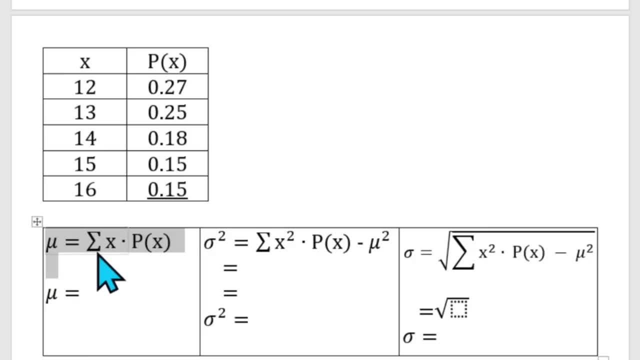 And it is determined by finding the summation of the product of the sum of the products of the possible value at its corresponding probability. While the variance is denoted by lowercase letter sigma, squared equals the difference between, here, the sum of the products of the squares of the possible value at its corresponding probability, and the square of the mean. 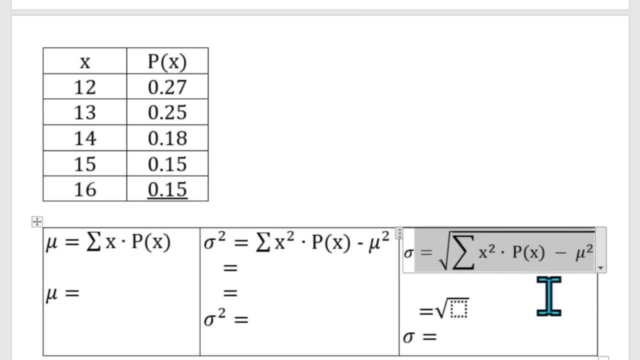 While the standard deviation is simply the square root of the variance. Let us proceed to solve this problem. The first column again are the possible values. The second column are the corresponding probabilities. Let us add another column here And we will denote this as the product of. 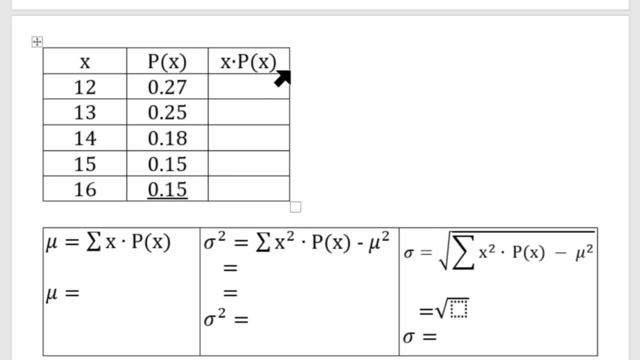 as the product of the possible value and its corresponding probability We have: 12 times 0.27 is equal to 3.24.. 13 times 0.25 is equal to 3.25.. 14 times 0.18 is equal to 2.52.. 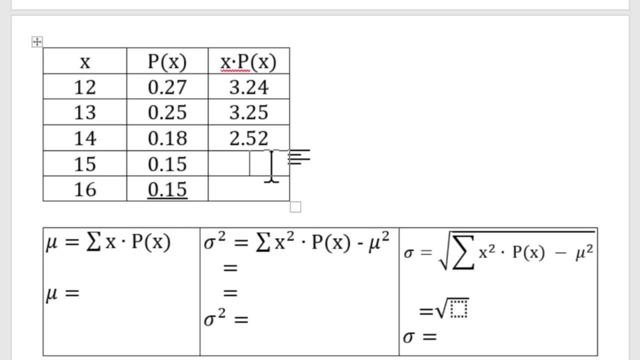 While 15 times 0.15 is equal to 2.25.. And 16 times 0.15 is equal to 2.40.. We now have the products of the possible value and its corresponding probability. Next is we determine the squares. 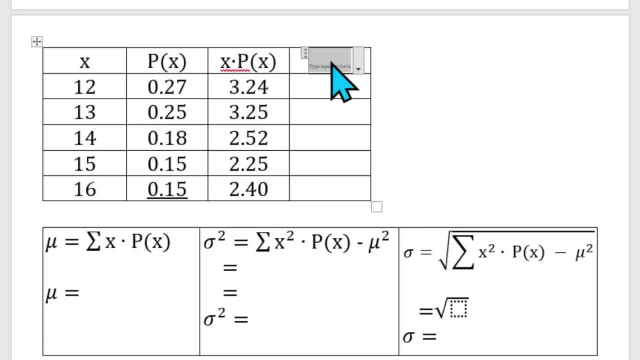 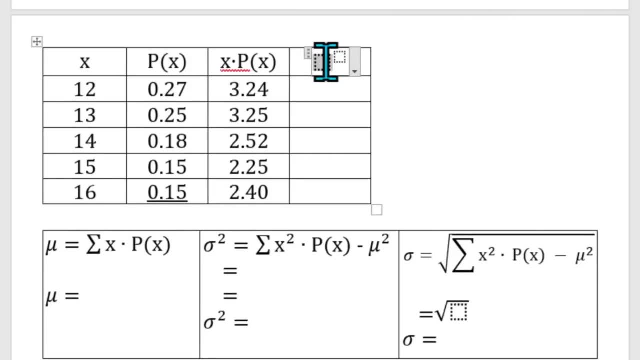 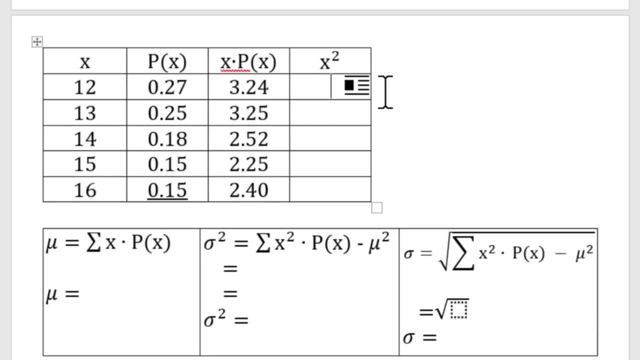 We add another column And determine the squares, The squares of our possible values. We have x squared And we have 12 times 12, or 12 squared is 144.. 13 squared is 169.. 14 squared is 196.. 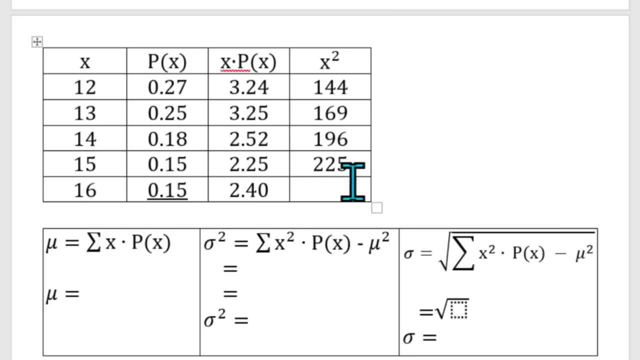 15 squared is 225.. And 16 squared is equal to 250.. After this, we need to add another column in our table And we label it as the product of the squares of each possible value and its corresponding probability. And we label it as the product of the squares of each possible value and its corresponding probability. 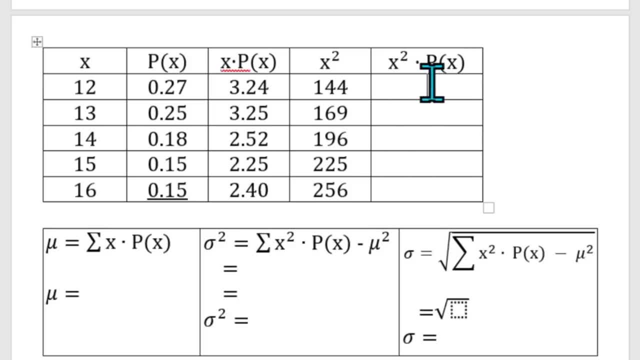 Okay, there you go. Okay, there you go. We have x squared the square of the possible value multiplied by its corresponding probability. We have 12 times No, we have 144 times 0.27.. And that is equal to 38.88.. 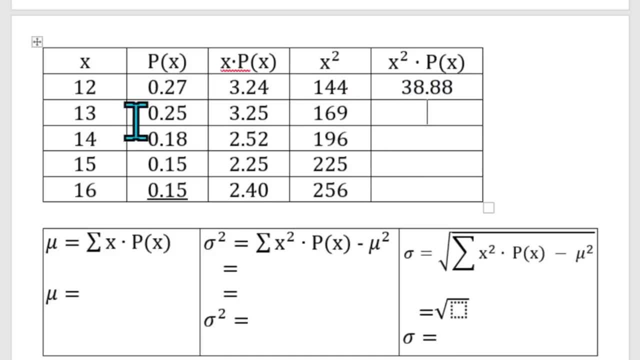 Next is: 169 times 0.25 is equal to 42.25.. Next is 0.18 times 196. And we have 35.28.. 225 times 0.15 is equal to 33.75.. And lastly, we have: 256 times 0.15 is equal to 38.40 or 4.. 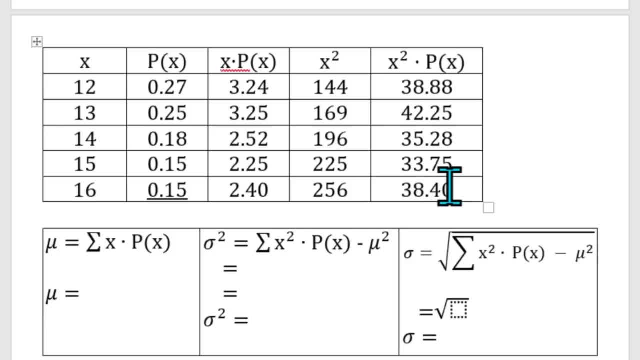 And, lastly, we have 256 times 0.15 is equal to 38.40 or 4.. Now that you have these values, we can now proceed to determining the mean and the variance and the standard deviation. Now that you have these values, we can now proceed to determining the mean and the variance and the standard deviation. 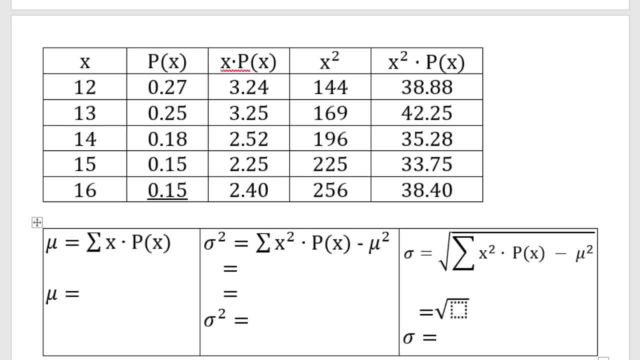 Let us first have the mean. Again, the mean is denoted by the summation of the products of the corresponding values. Again, the mean is denoted by the summation of the products of the corresponding values. Again, the mean is denoted by the summation of the corresponding values. 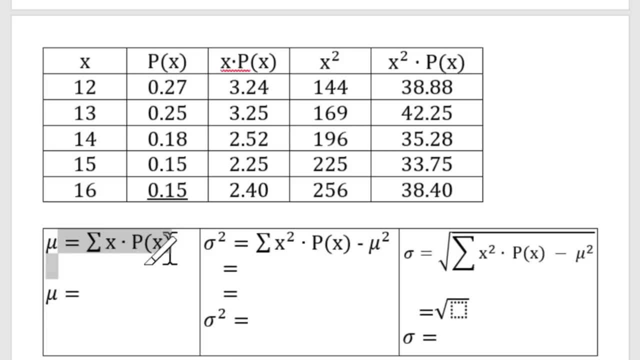 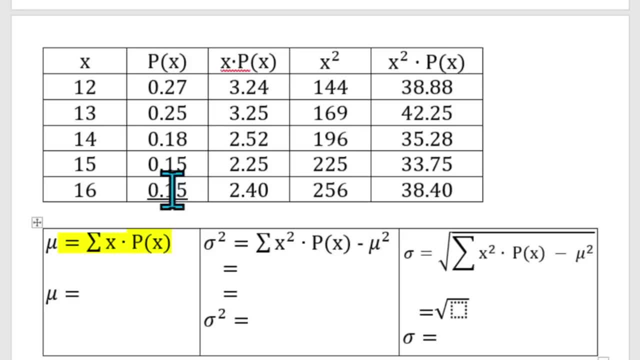 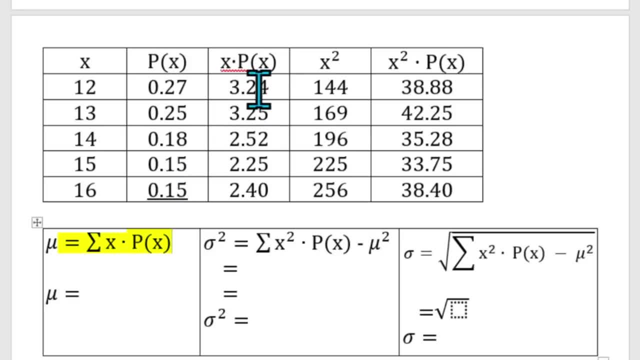 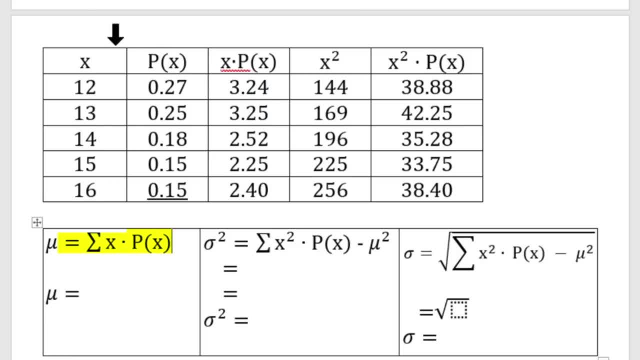 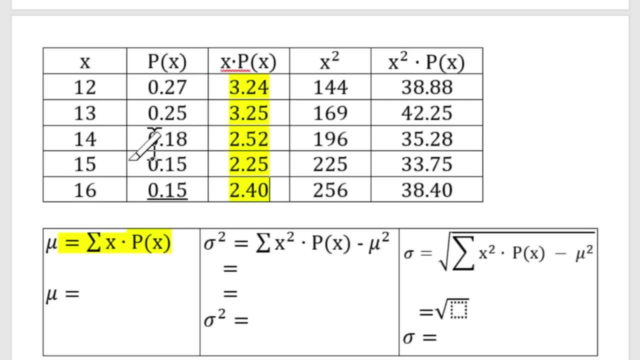 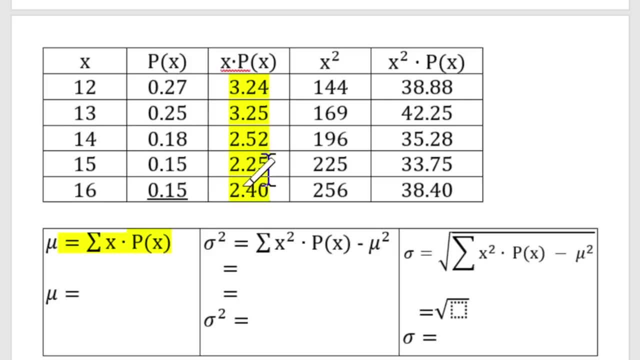 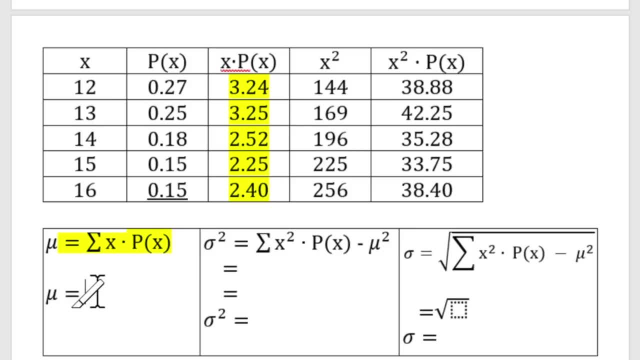 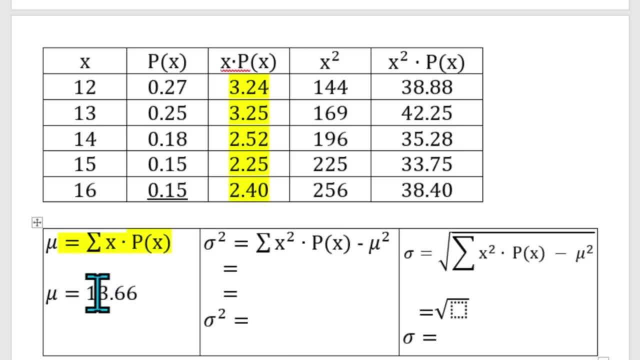 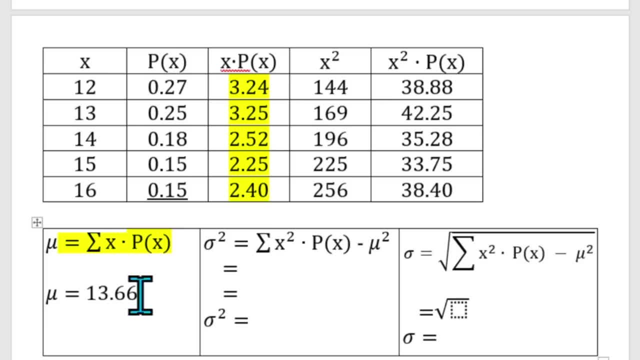 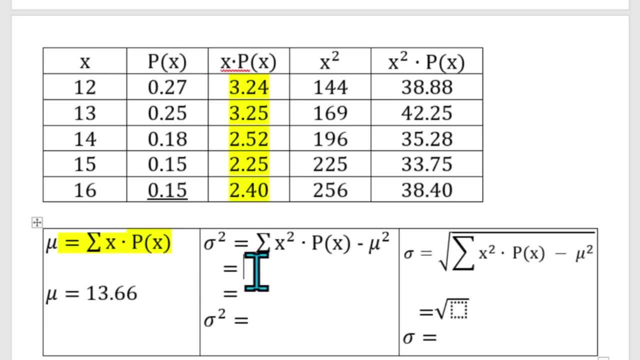 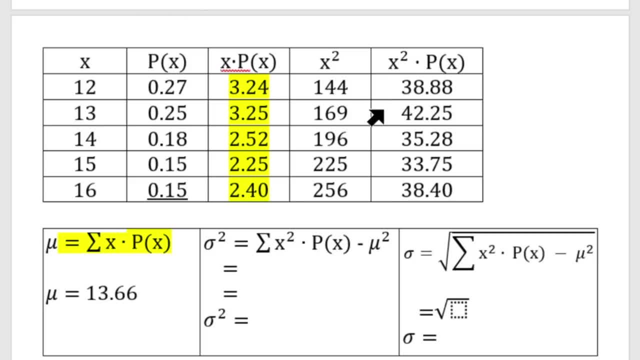 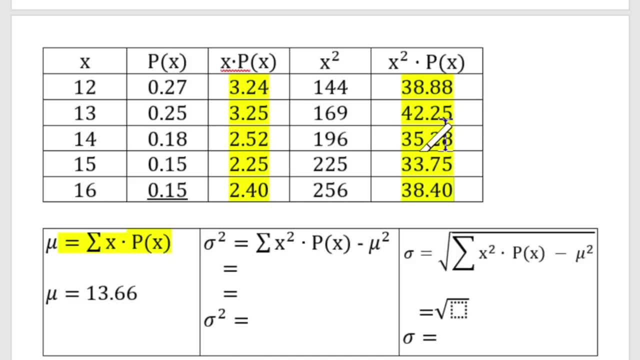 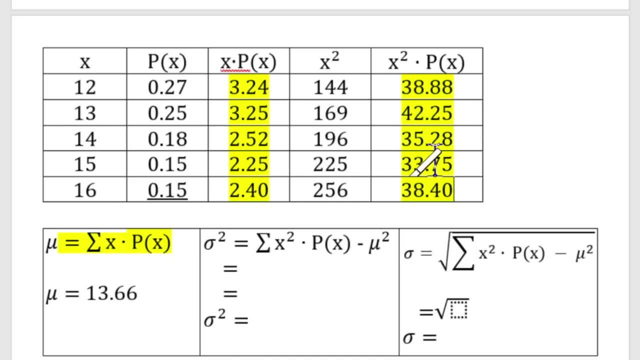 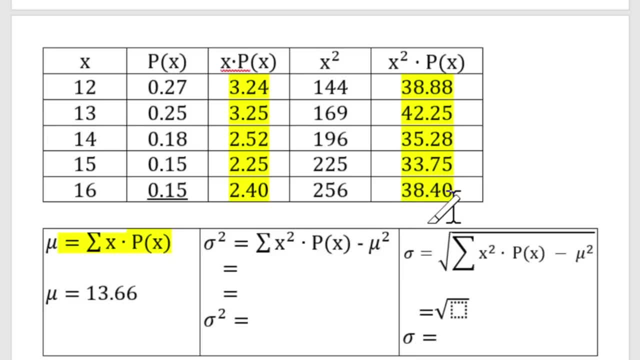 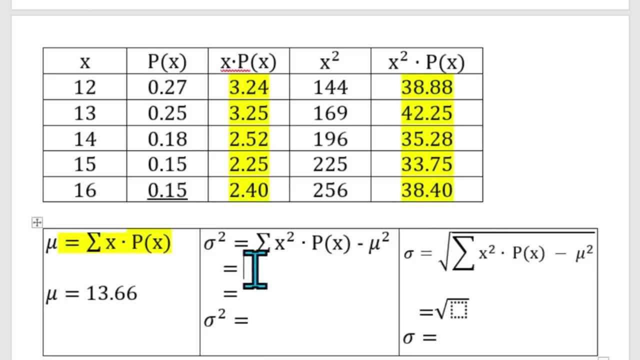 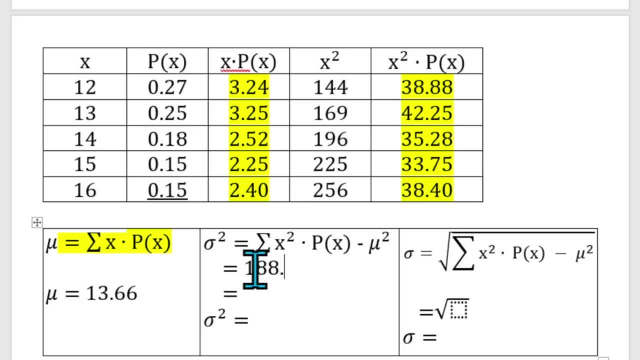 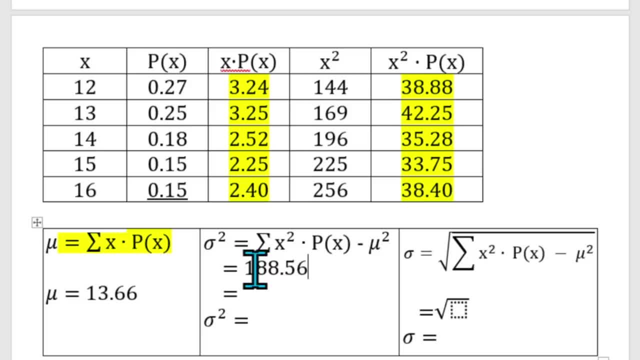 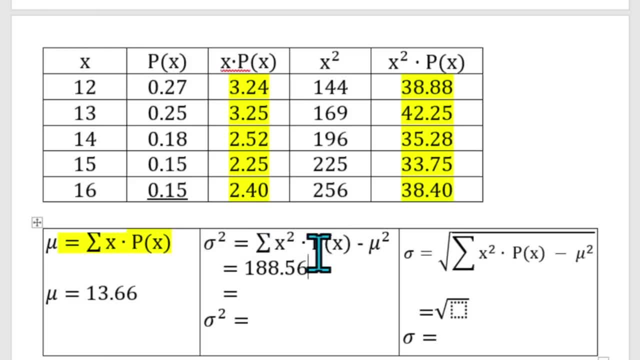 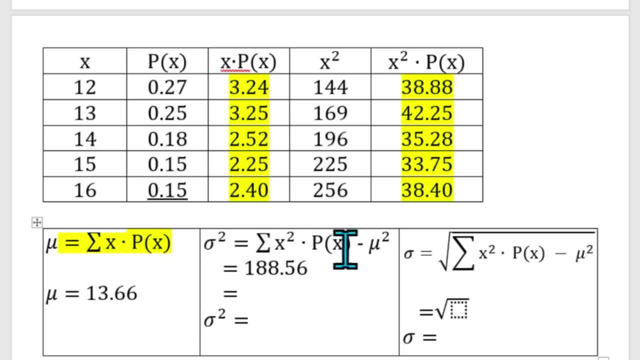 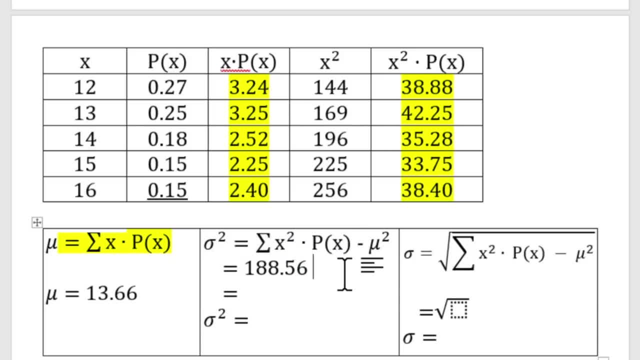 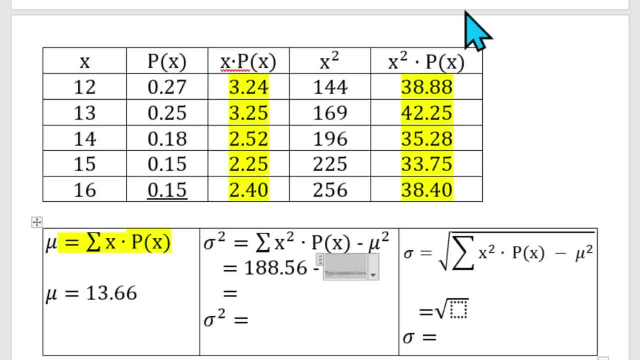 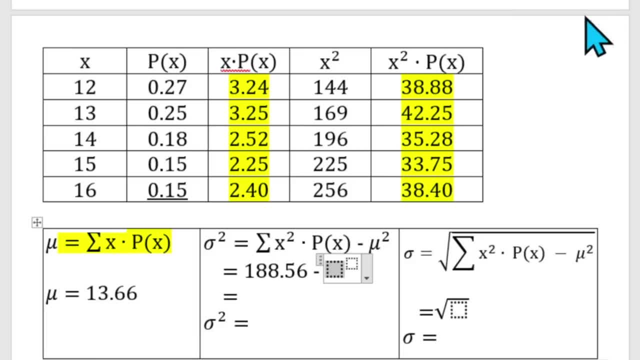 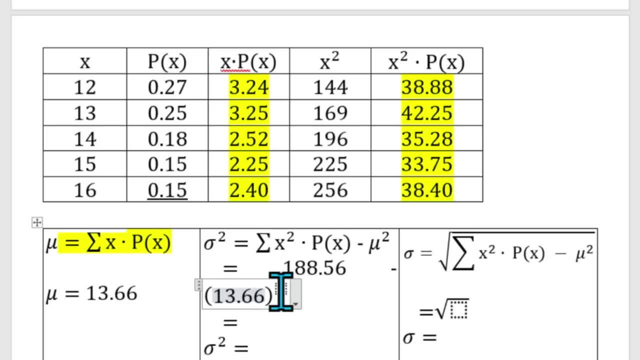 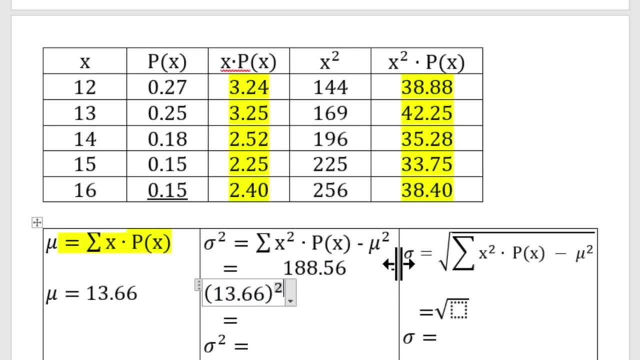 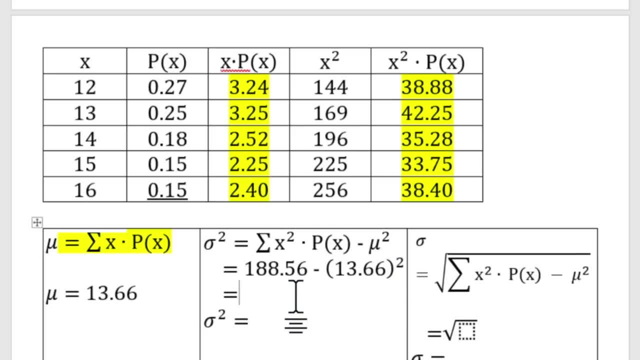 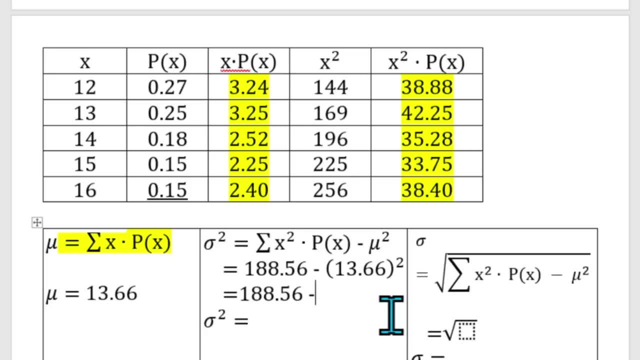 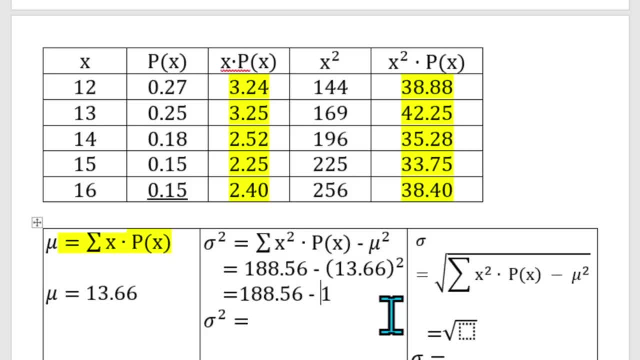 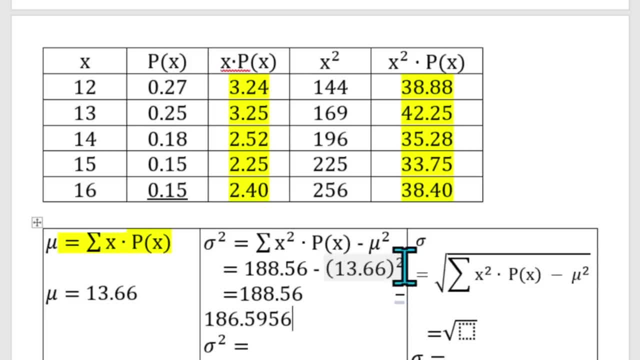 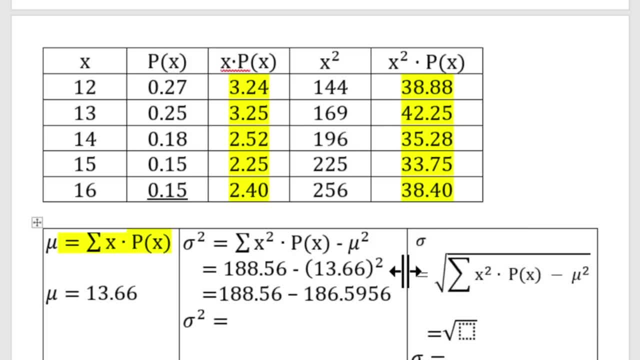 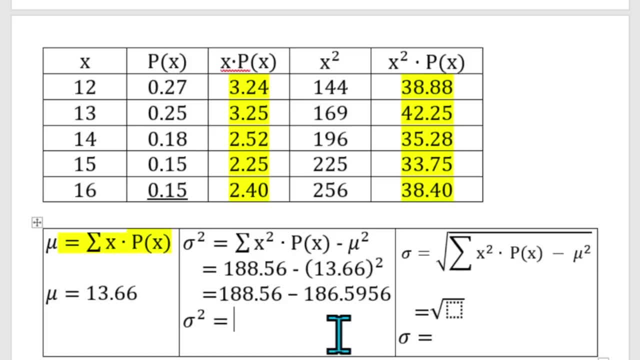 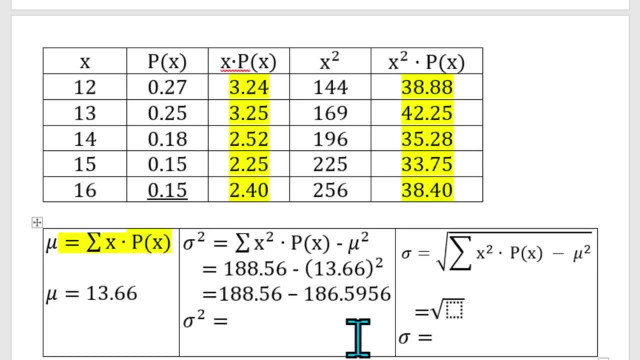 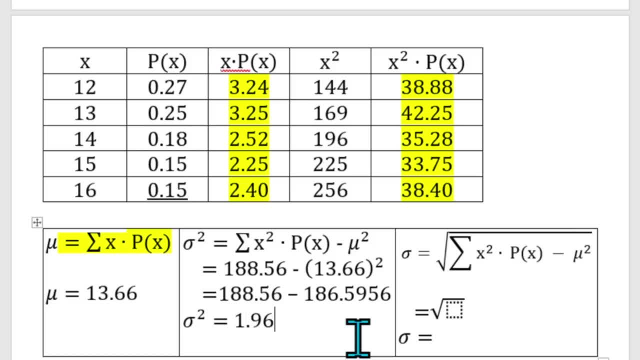 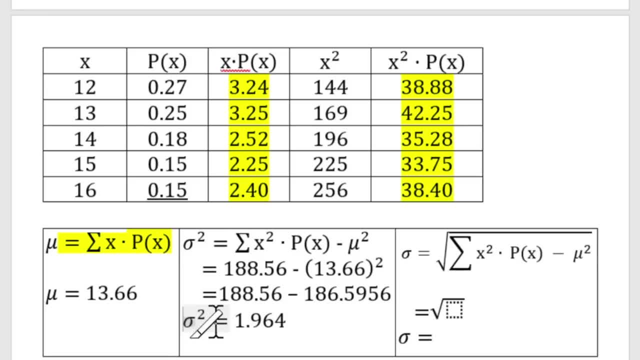 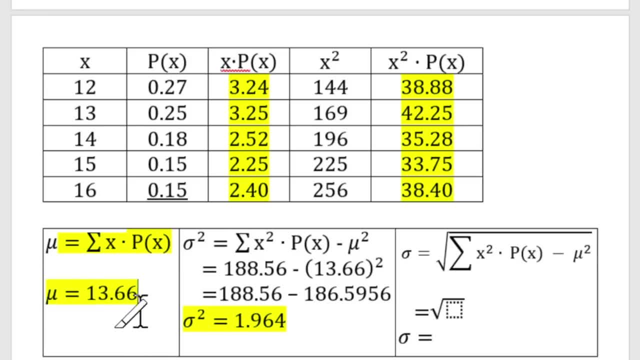 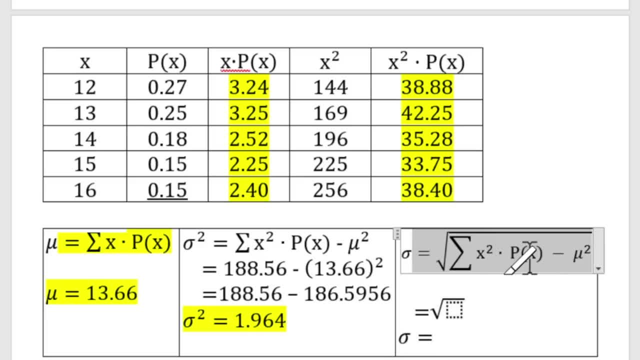 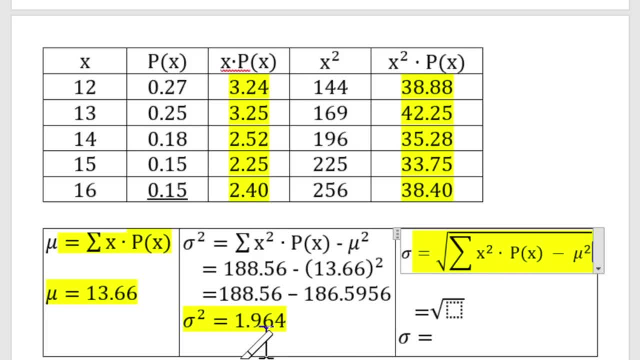